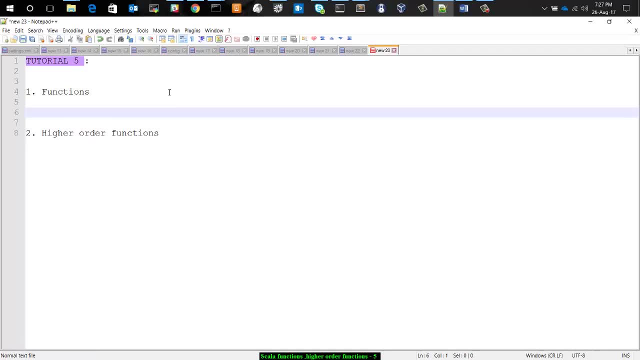 of function def. This is how we define a function in Scala: Function name, then parameters: default return type. Function name, then parameters: default return type. Confirmation of function value: default return type. Let's give a hint: Function name, then parameters: default return type. 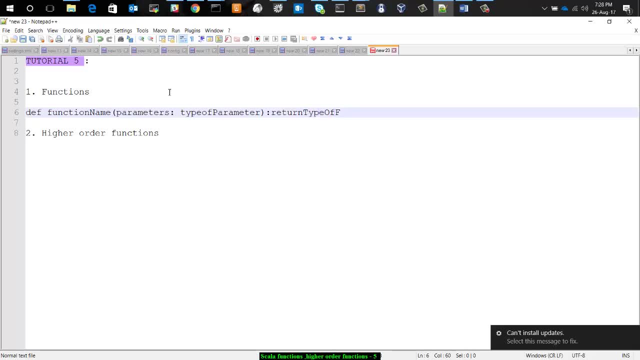 Function name in the above syntax operator is like a returning or assigning the value. you can create function with or without this equal to operator. if you use it, function will return a value. if you don't use it, your function will not return any values. let's get into an example and write an example with this equal to operator and: 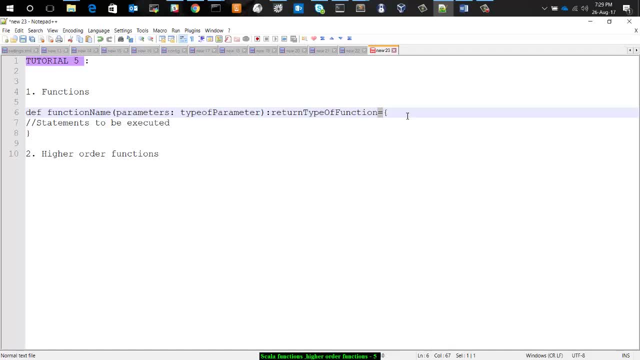 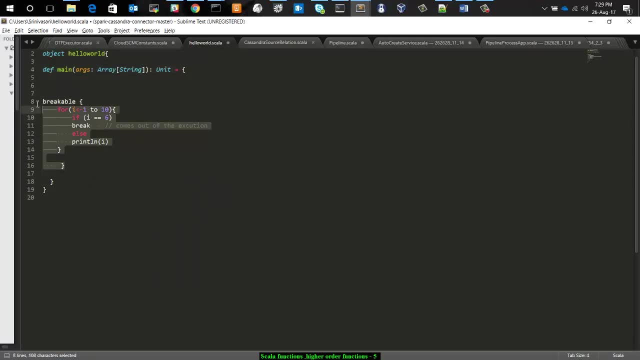 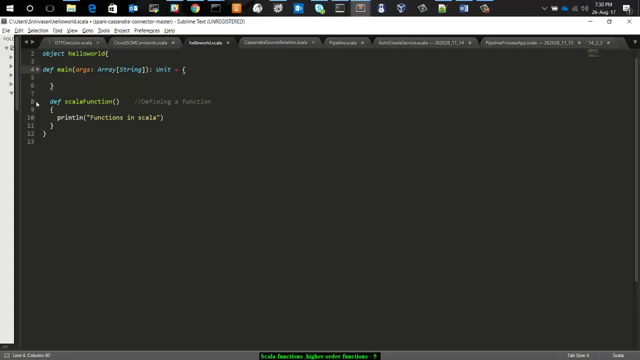 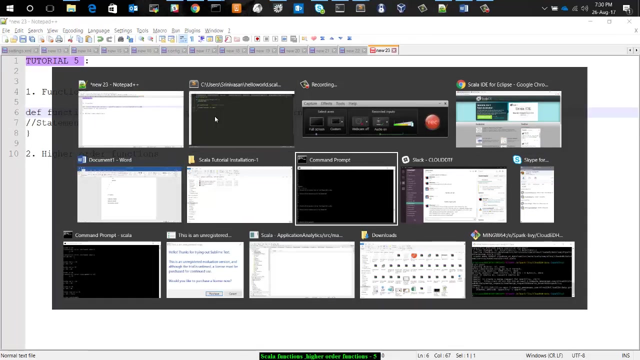 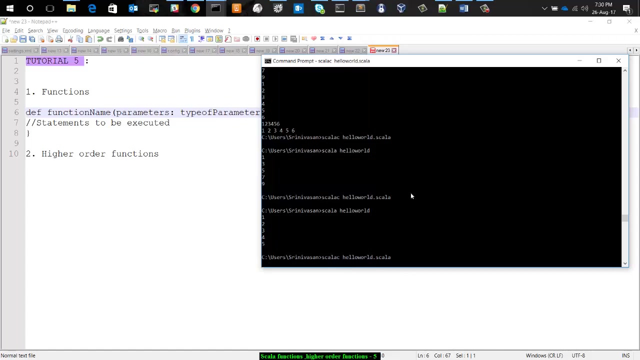 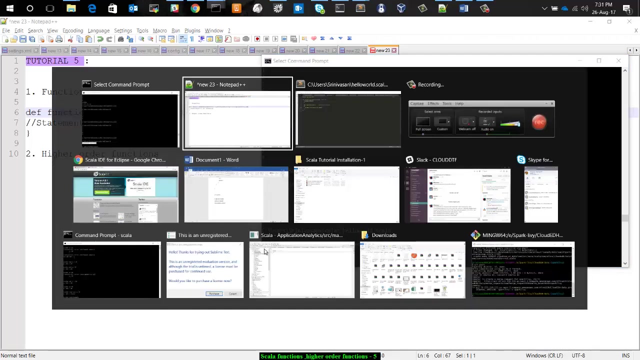 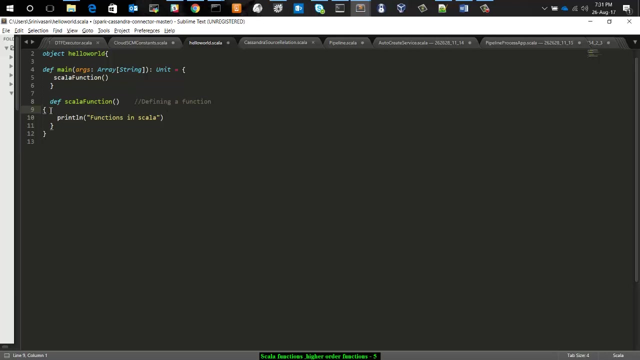 defined in a function, and here i'm going to call that function a function, as j answering the function. Let's see the output of this function. You can see that it returns correctly. Then we can write out with an equal to operator. If you give an equal to operator over here. 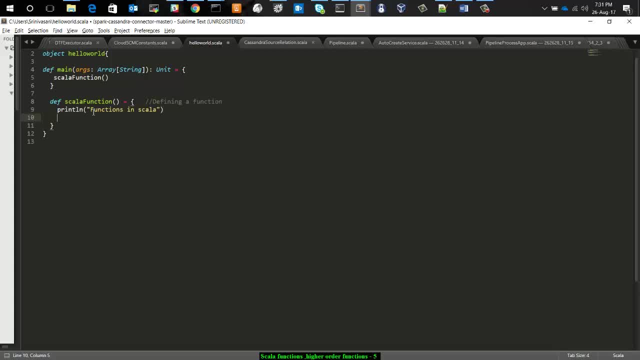 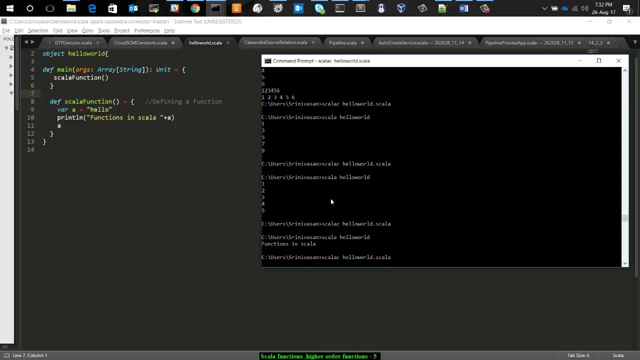 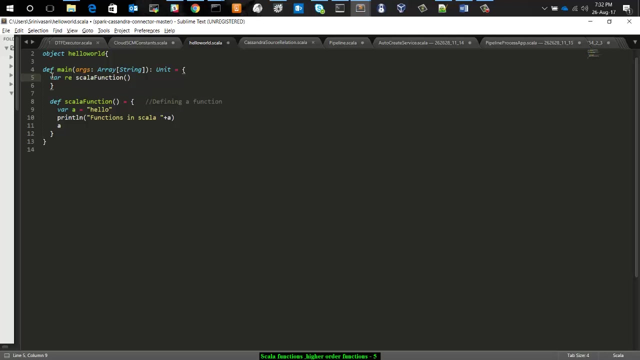 It means the function is going to return something. Ok, So we have to give a return something. Hello, Let's save it and check out. Ok, You can see that it works correctly. Then we need to check whether it is returned correctly or not. Right, So I am printing this: 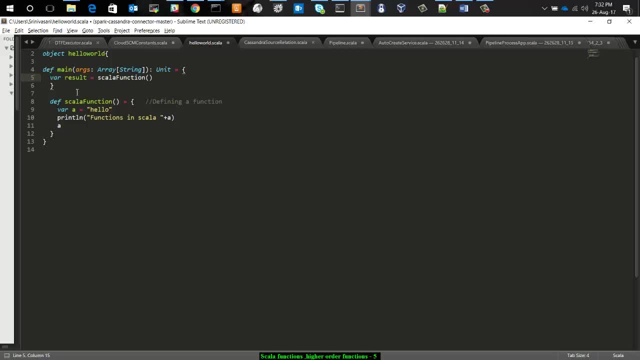 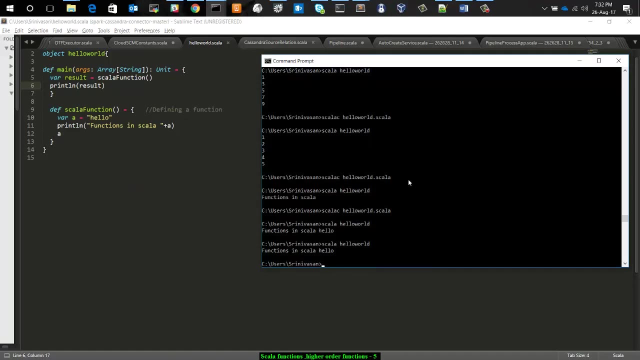 Print this KLA function And saving it in here. Then I am printing the result And saving it again. Let's check. Sorry, We need to compile it first And then run it and check it. It worked properly. You can see that the data value has been returned from the function. 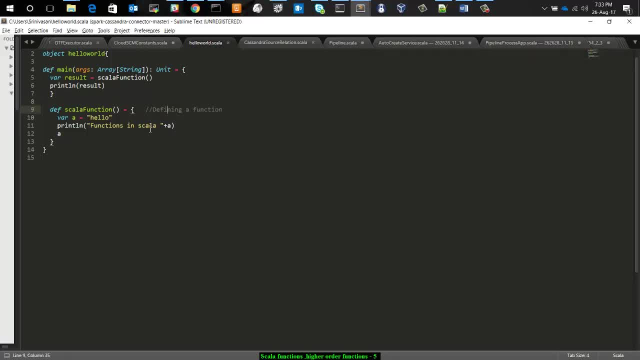 Now let's see how to give a parameterized function in KLA. In here I am declaring an int and p, Which is also an integer, So I am going to give a parameterized function in KLA function. So I am going to give a parameterized function in KLA function. 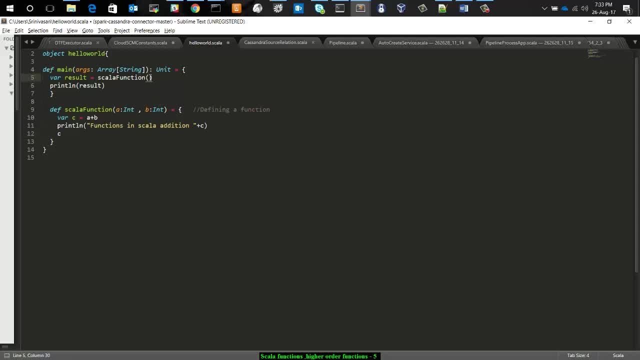 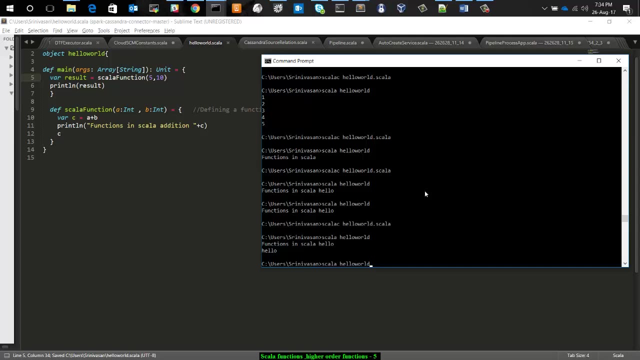 And here I am returning a value as C10. I am passing this to integer 5,10 And I am saving it over here. And let's see what's the output of this one. And here I am passing a value as 5,10 And I am saving it over here. 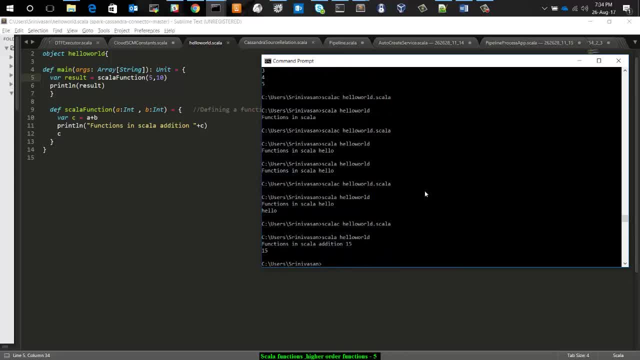 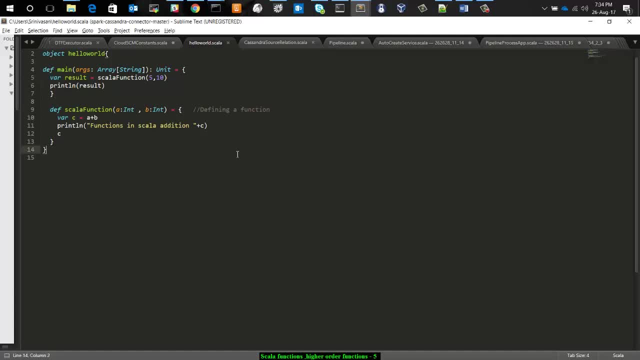 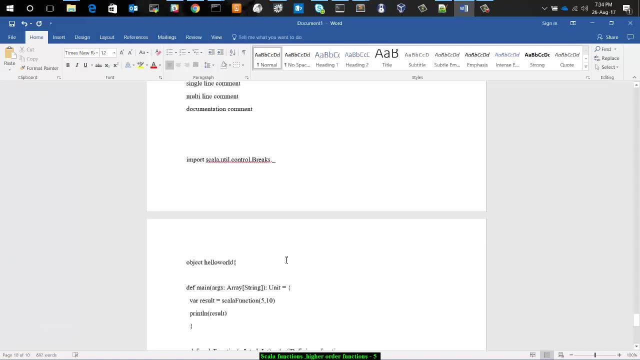 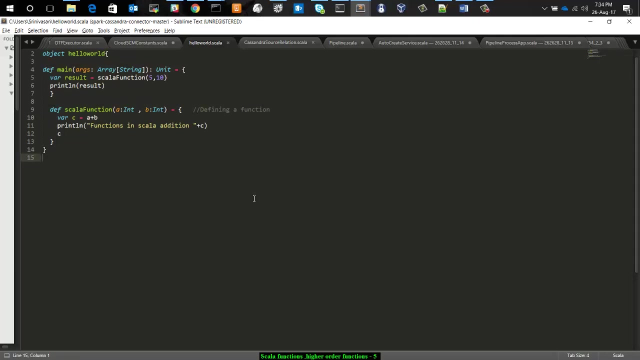 And let's see what's the output of this one. If you can see this, it contains it clearly. It returns the output as characteristic given in paramseceptor. Let's see how to do the rec向 function. I am going to recommend toomsluger RC Tyler. 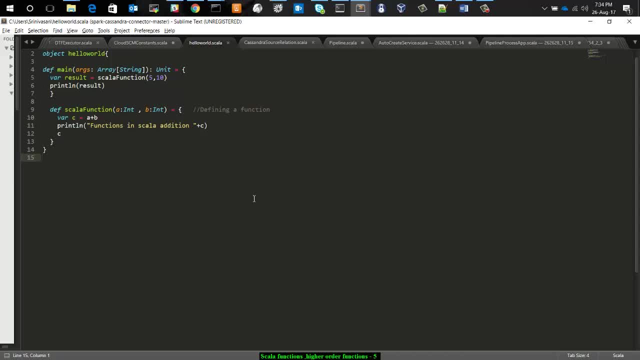 And let's see what's the output for it. I'm going to write one program which is going to multiply two numbers by using recursive function. You can create recursive functions. Be careful while using recursive function. There must be a base condition to terminate program safely. 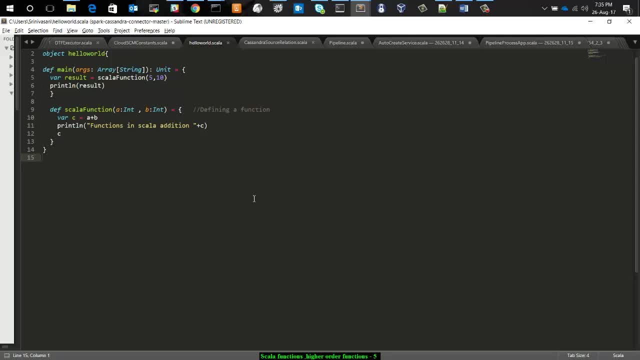 Let's see how to write a function I'm returning. the return type of this function is integer. I'm writing one condition: If a equal to zero, This should be the condition. It returns zero, or else A plus function. Let's see. 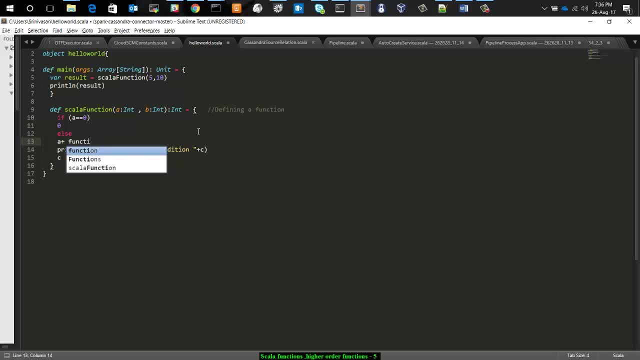 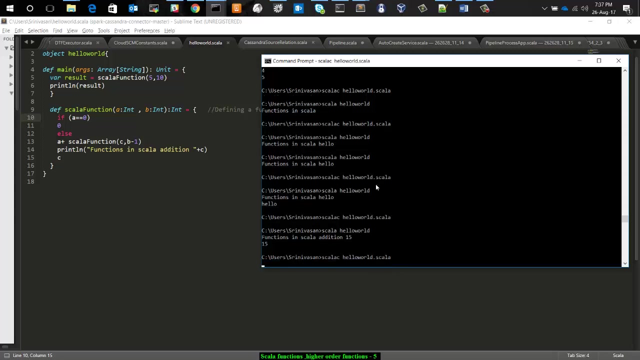 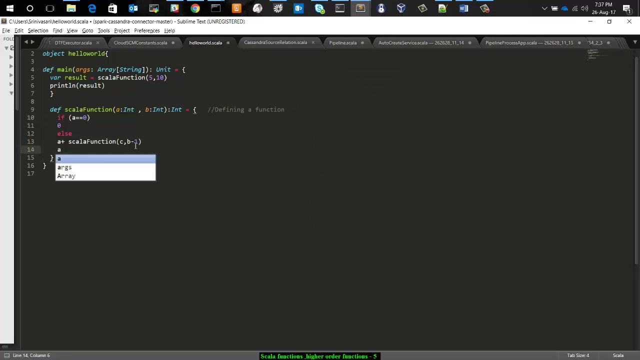 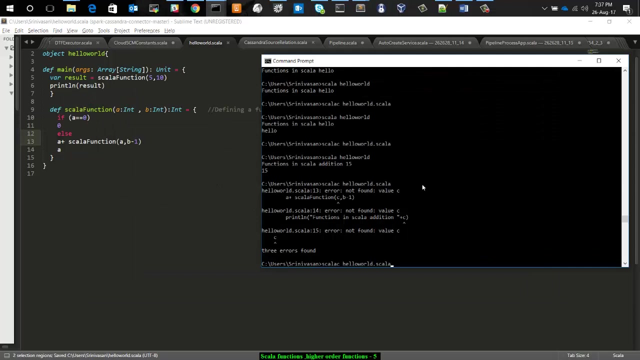 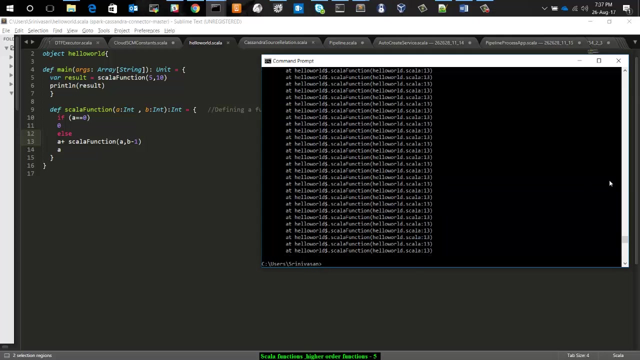 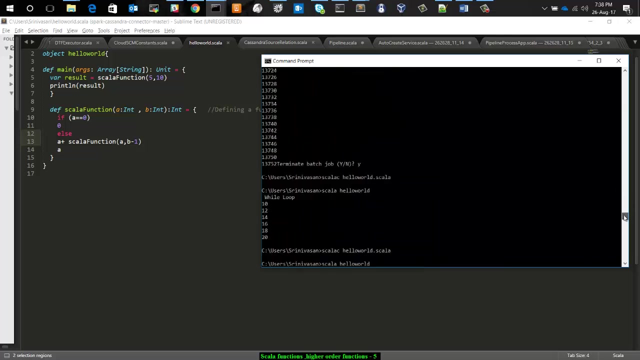 Let's see function. Let's see that function. Let's see, Let's see, a minus 1.. Let's check, look how it works. I'm saving it, OK, OK, OK, OK, and find another. so what it does is just print out. it just called the function 30 times. 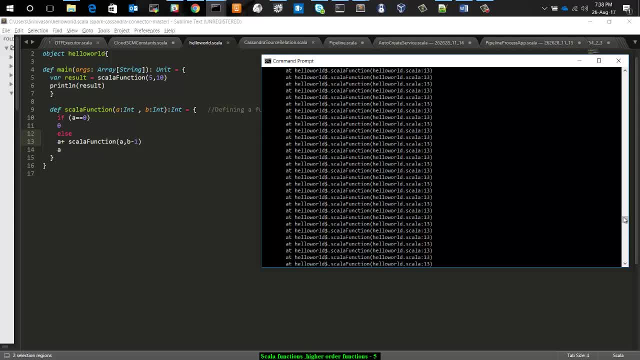 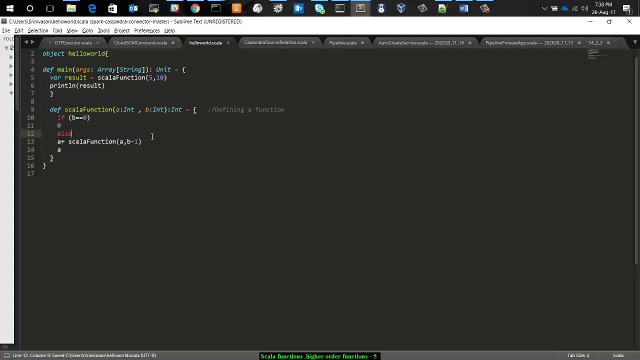 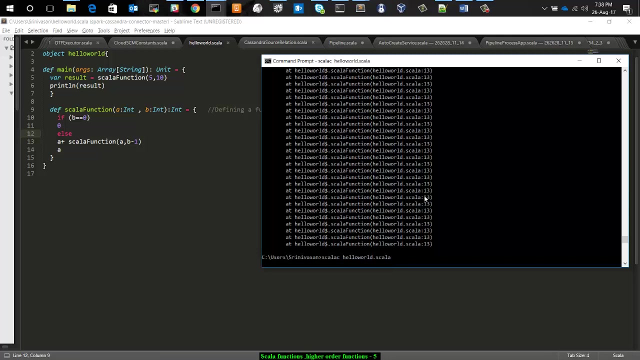 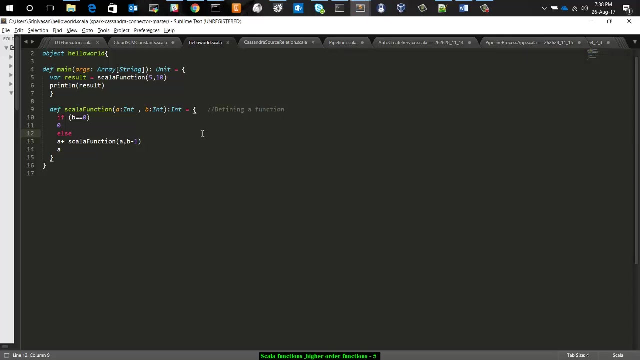 oh sorry, it has some stack overflow error. let's see why throws this here. the value is five. now let's see how to how to work with the function. it's a, a default value deeper and the default value is nothing, but these values will be defined with them by its default value is zero. is how we need to define. 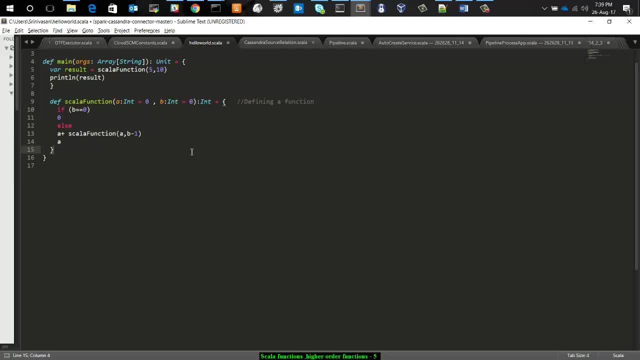 the default value of the program by equating it with zero. then we can also pass a variable name along with the parameters. while calling a function like in here a is equal to five, in here the is equal to 10. so that chemical name like called function a was tested as to how toétique functions. hours. 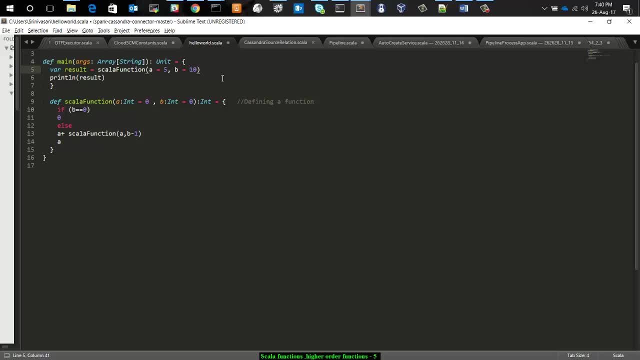 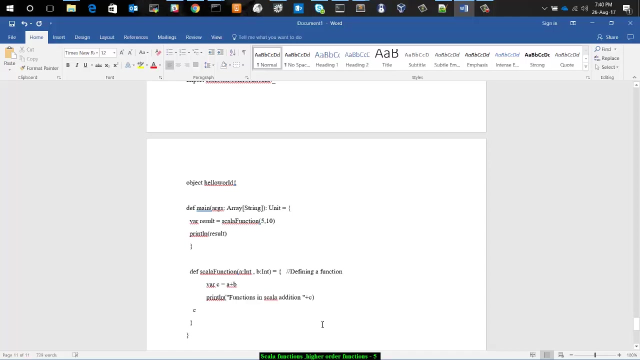 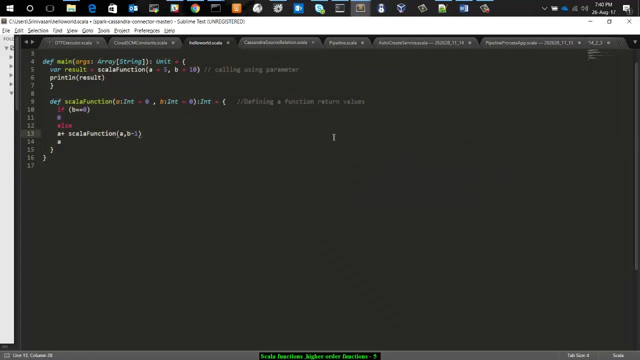 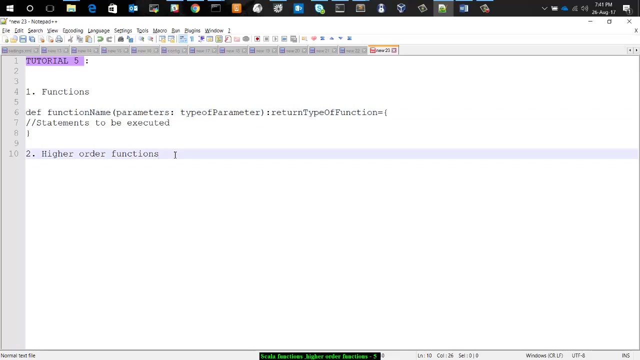 that on the other common example i called, function in with function b is equal to 5 for final display bar. it will be easy for us to clarify which which thing we are calling only using parameter. so values, okay, we don't need to. the next, the next topic we are going to see about higher order functions. higher order function. 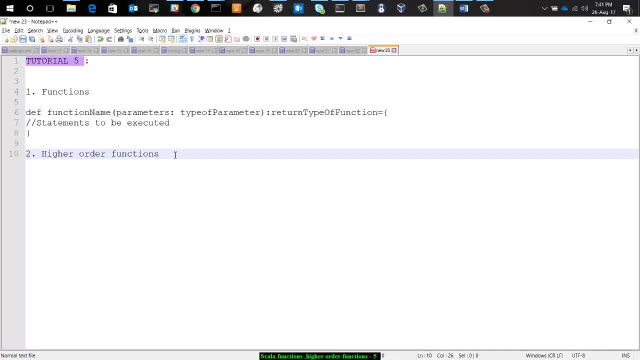 is a function that either takes a function as an argument or returns a function. in other words, we can see the function which works with the function is called higher order function. higher order function allows you to create a function, composition, lambda function or random as function. uh, usually, um, while calling a function, we can pass as a function in uh to other other. 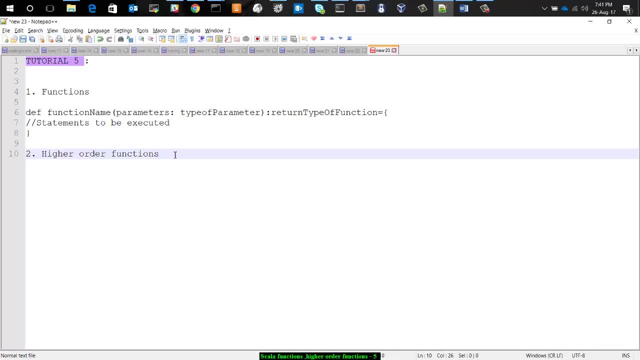 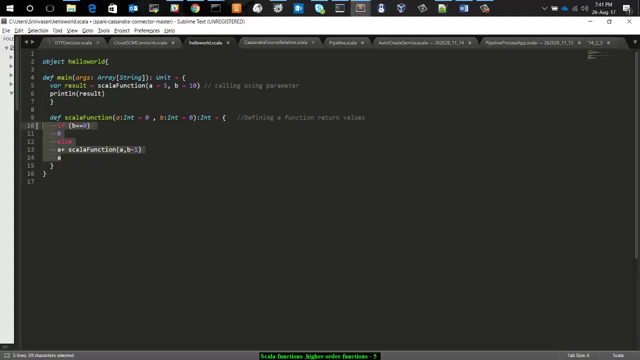 function as a parameter. let's see a scalar example: how to pass a function as a parameter in a function in another function. let's see there is a main function, another function is there, so so the output of this can be anything and it's going to return nothing. 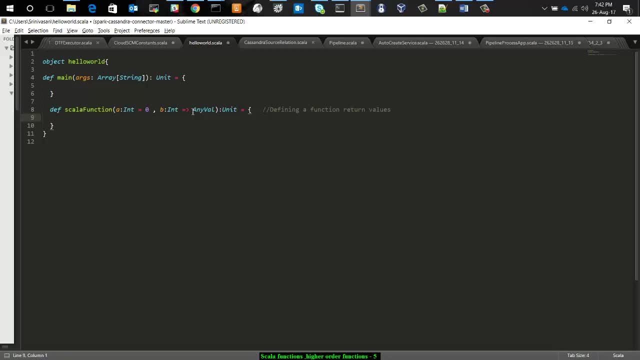 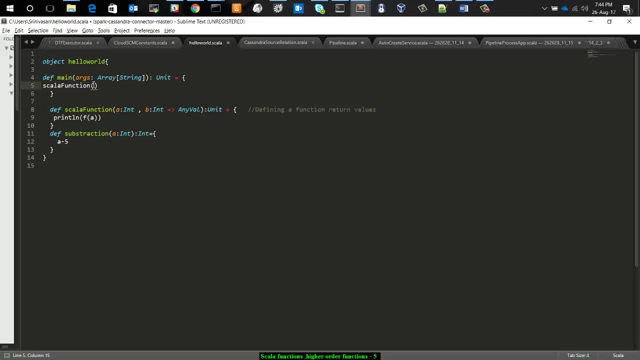 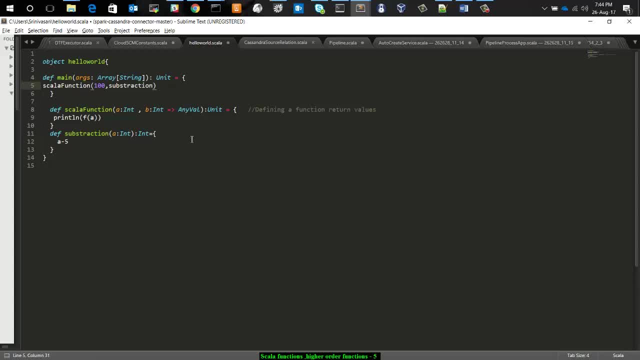 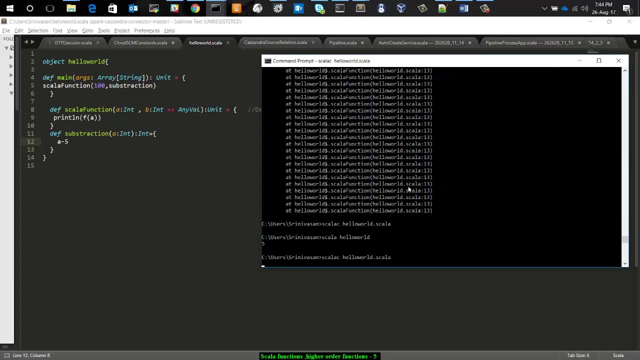 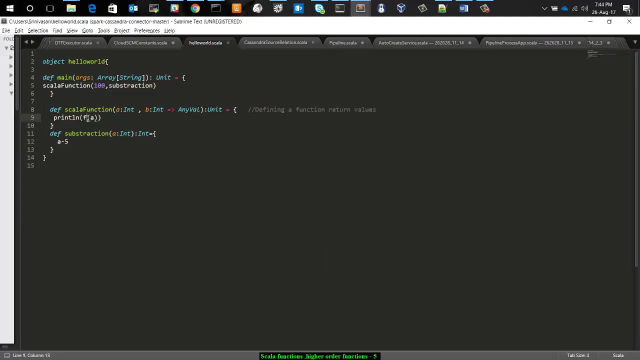 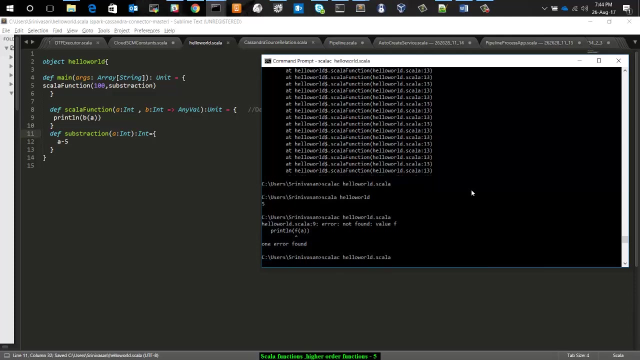 let's do a simple subtraction. let's do a simple subtraction, Save it and let's see what the output it gives. it looks like a not found value f of a. sorry, Now returns. it gives the correct answer. you can clearly see this. I have written a. 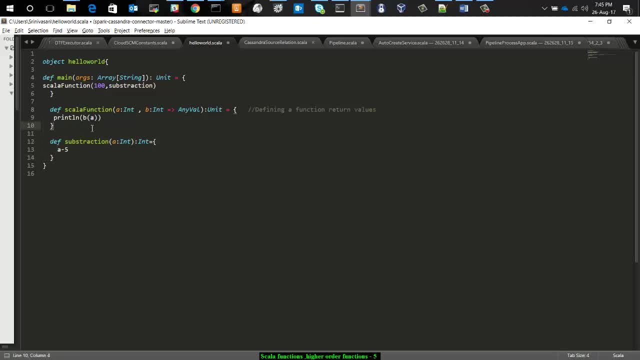 subtraction as involved one function and the scalar function, which is going to return any of the values. So I have called this function in main method and passed this function as another variable, which means I am going to assign this b for another function and this function is going to return any value. 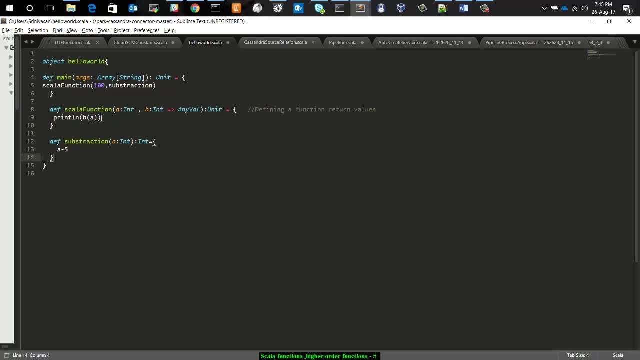 and it's getting saved and it's going to throw output which was decided by us. Now let's see the function again: Function composition function. function composition functions can function can be like, it can be composed from other function. It is a process of composing in which a function represent applications of two composed functions. 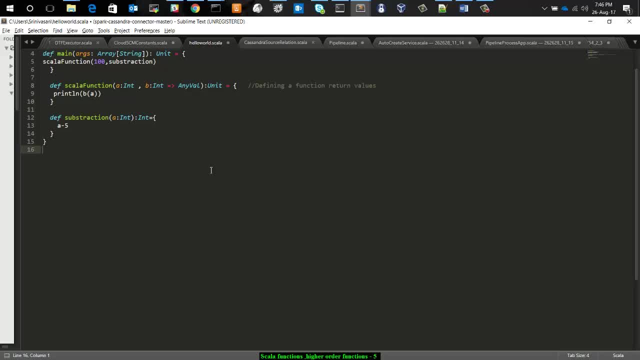 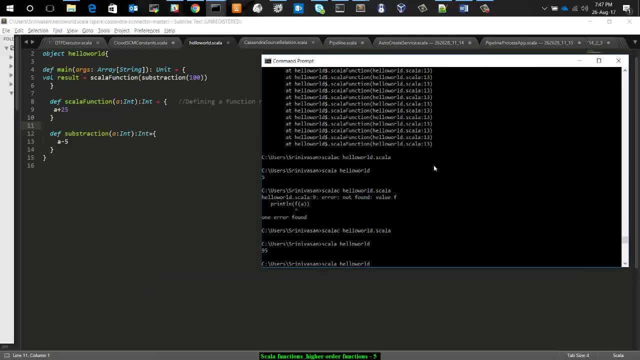 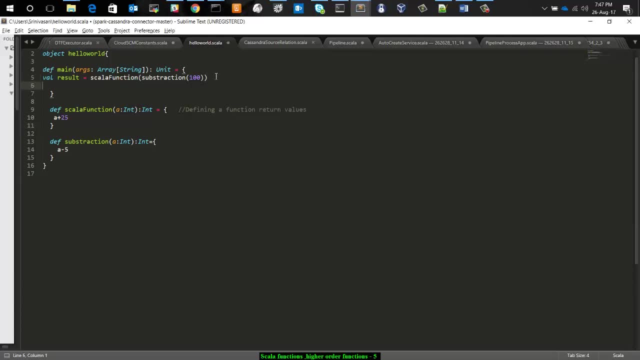 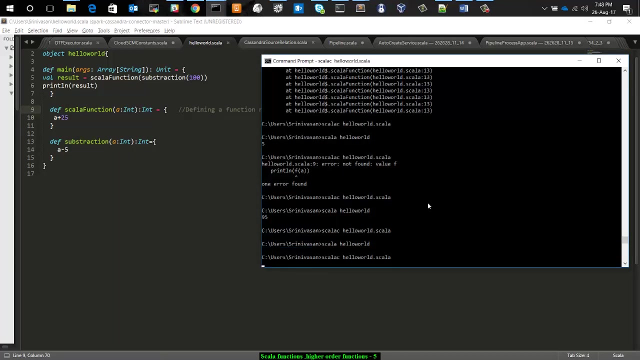 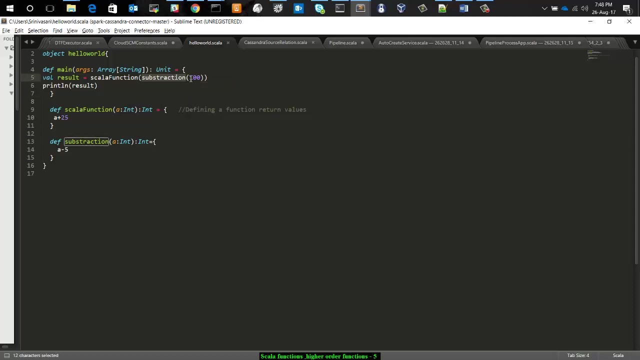 And let's check what's the output of this one. Oh, I forgot this. Print this result. Print this result. What it does is I'm calling a function and passing a function of another thing. The first what will work is I'm calling a subtraction function which is going to minus 5 from 100.. 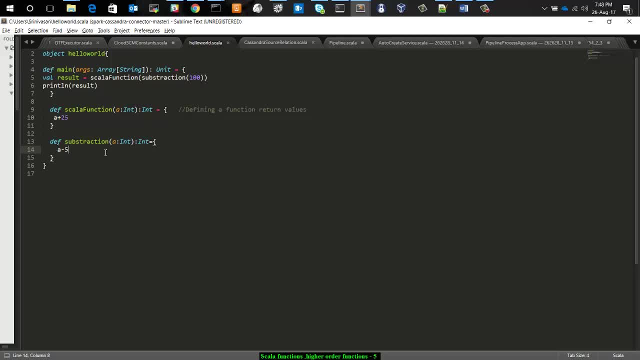 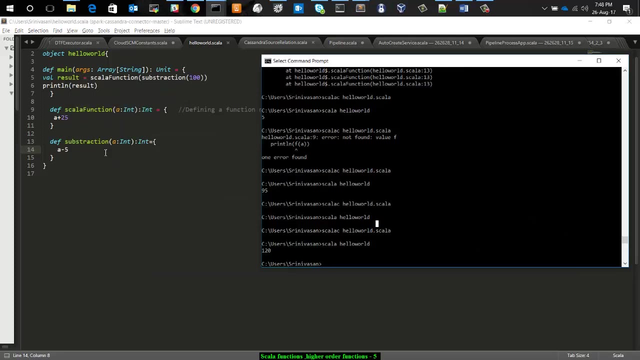 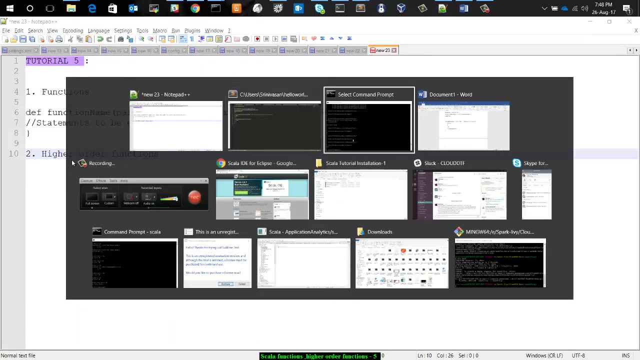 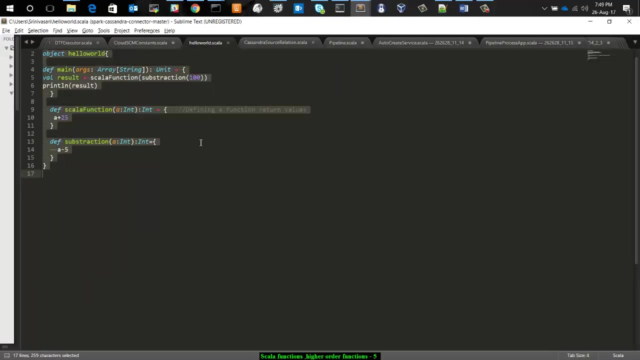 And then the return type of this is going to scalar function which is going to add plus 25 to it And return the value and saving it. in result And printing it, The value is coming as 120, which is correct. Then in functions in scalar there is one special type of function known as lambda function, or it may be called as anonymous function. 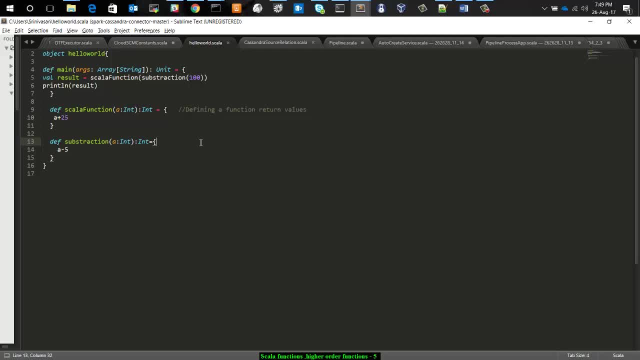 In this function. it has no name, but works as a function. It is good to create an anonymous function when you don't have to use the same function again. Let's see how to write this anonymous function here. Let's do it. 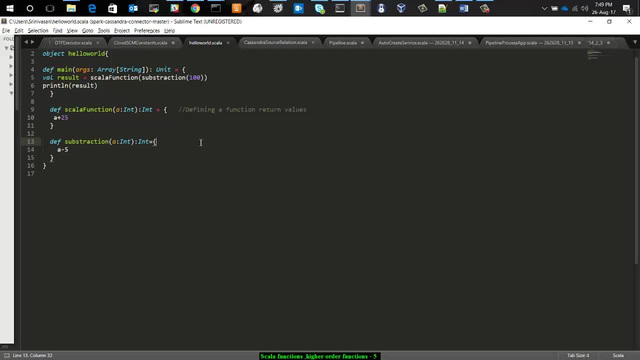 Let's go. this is known as an anonymous function. this symbol is known as the rocket symbol in Scala. Now I'm creating another one result which is underscore, me underscore, and I'm typing integer, which means it a n is a n is a n is a n. 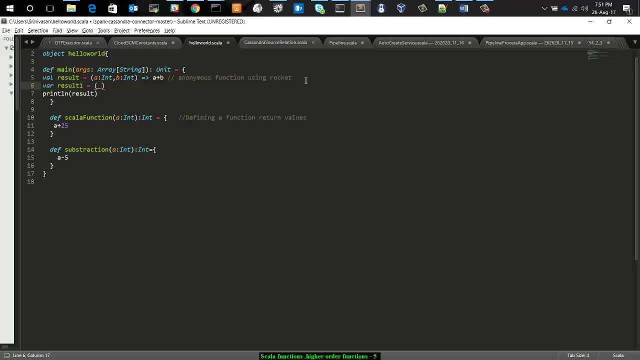 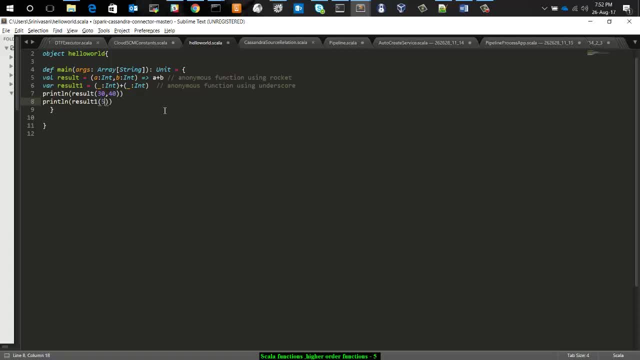 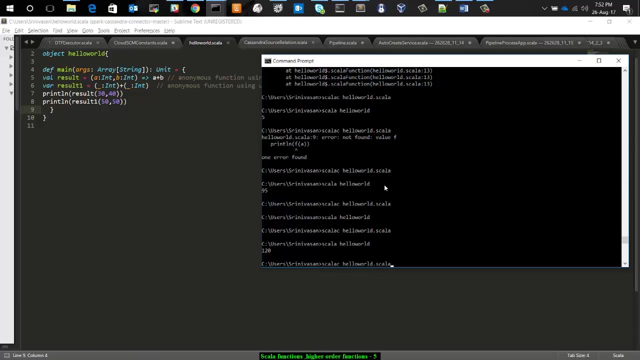 I'm saving this and let's see what you get out of this program. you can see. you can see this: the first one throws 30 plus 40, 70, and the second second function throw. a second anonymous function throws 50 plus 50, which is 100. you can clearly see this. like both the things. 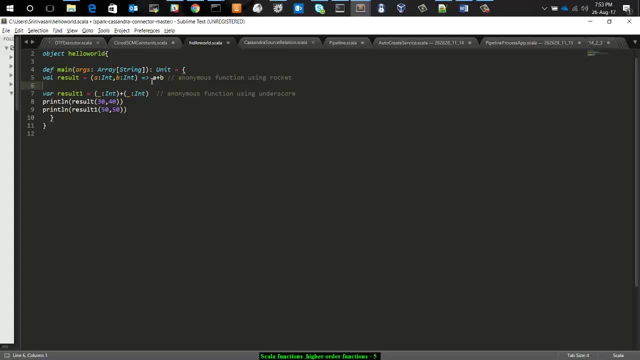 is correct. the only the way of defining this is different. in the first one we are using a rocket which is going to do as a plus b. in the second function it is going to take anything as an input, but it should be the type of integer. if you, if you pass pass string over here and try to run this program, it will throw. 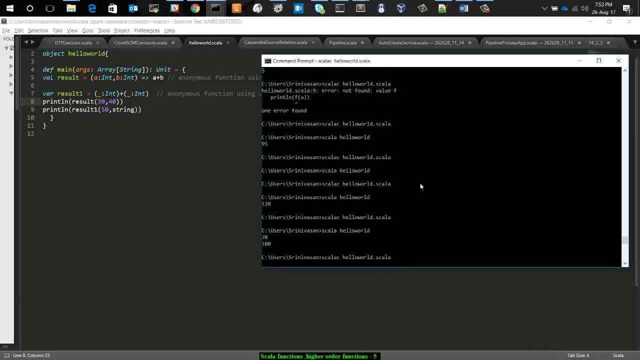 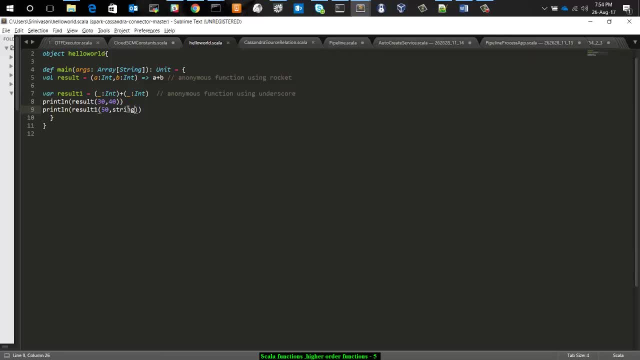 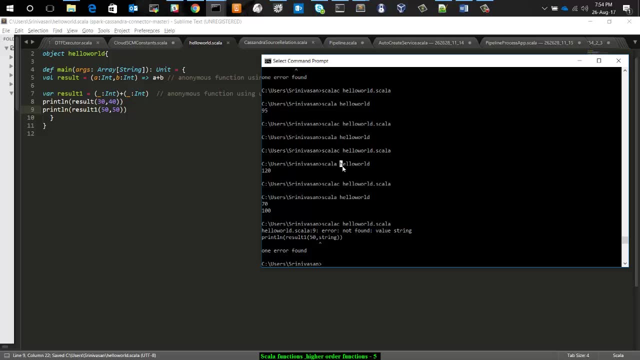 an error because of the type which we have defined in the program. you can see that one error found. the value is string, which is means the type is mismatched. so we change it, so we're gonna Save it and then we'll run it again. we are going to run this again. 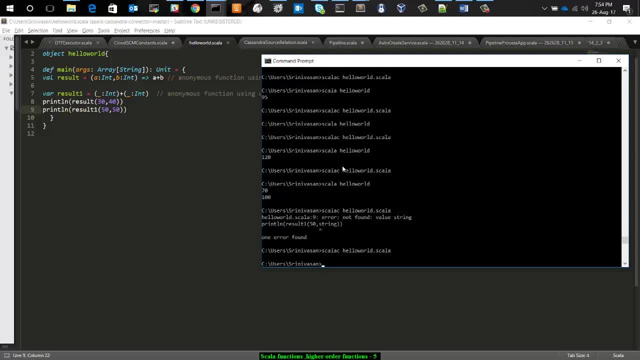 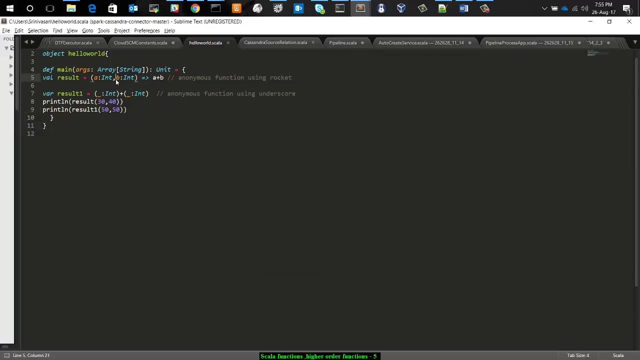 saveис, saveu, saveu, saveu, saveu e. as you can clearly see, the output is correct. and one more thing in scalar is: scalar can be defined in microline, which means this is how: if you go, if you define like this, however, it's going to take it in a correct way, but if you 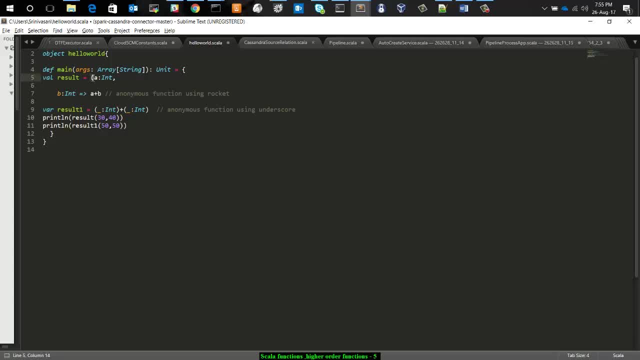 forgot to give this braces. it will throw an error that the function is not rendered correctly, so we have to give this one. this is known as multi-line expression in scalar. the next thing we have to going to see is scalar function carrying in scalar method. have may have multiple parameters. list when a method is called with a fewer. 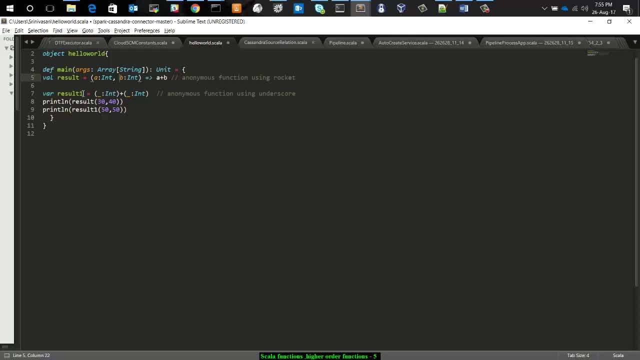 number of parameters list, then this will yield a function taking the missing parameter list as its arguments. in other words, it is a technique of transforming a function that takes multiple arguments into a function that takes a single argument. let's see an example of this one. here is an example of this real moment, when we're working with a real moment. 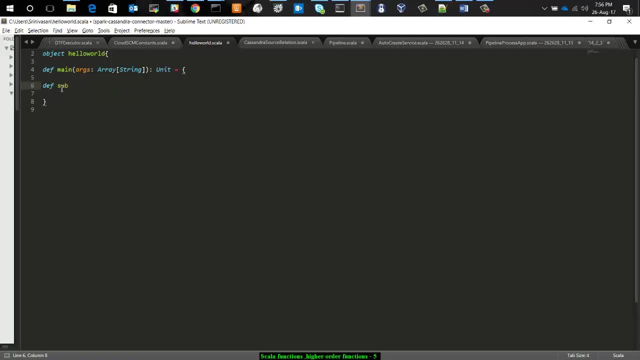 right now and we have a problem. actually, i have a problem with a real moment today. let's see what happens with a real moment. i'll explain. for example, let's say i wanted to give Вс a number of my once because i'm running my seminars at one point, so i spent my training during 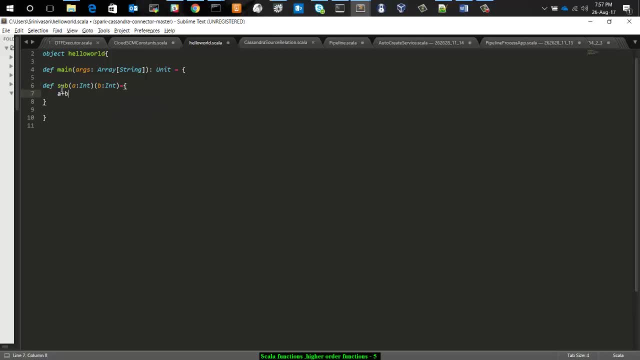 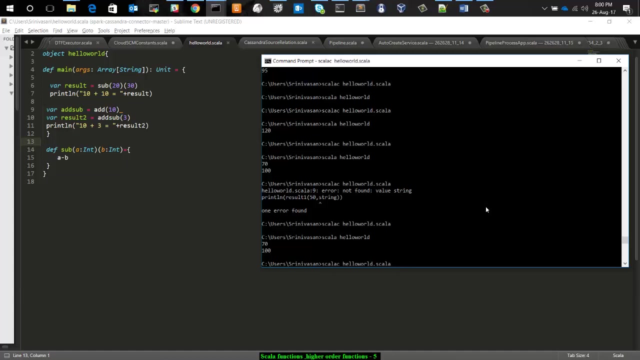 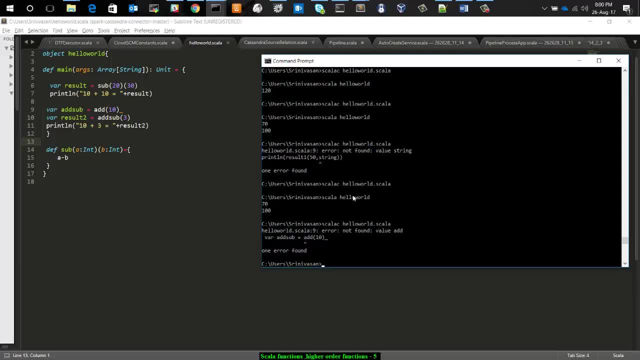 It shows like not found value add. Oh sorry, Let's see. Let's see. You can clearly see. this was the output of this program. The first one is like passing the two values using the curry function, which means the parameters which we are passing, is like a cutted one. 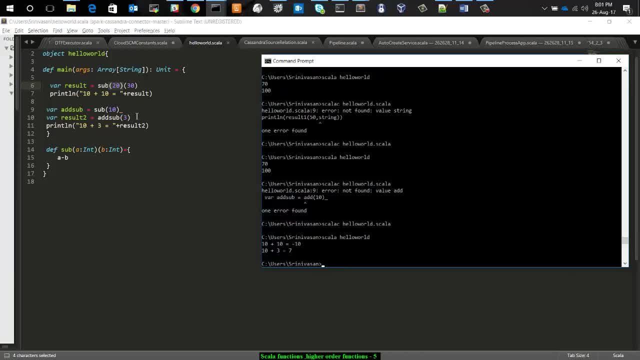 That's the first one, And the second one is like We are passing sub the first one first parameter and leaving the last parameter and saving it in add sub variable. Then in the second variable, result two- we are passing the second parameter. 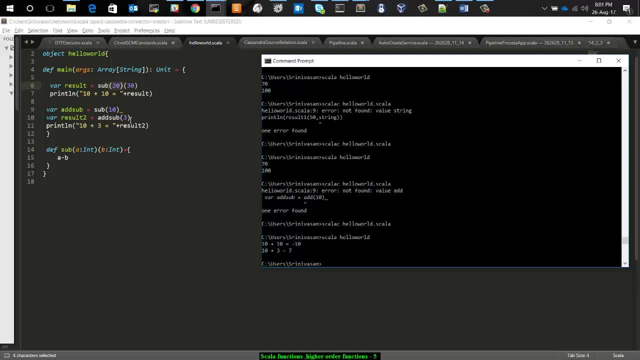 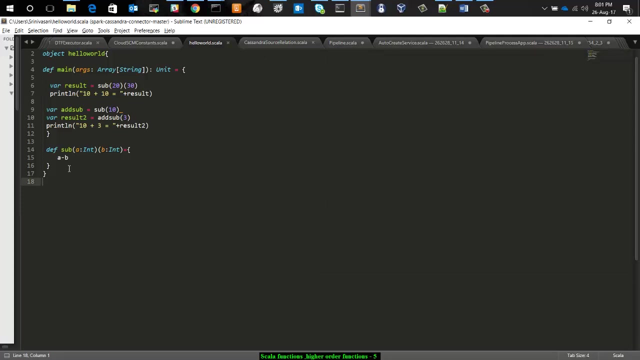 Now, while calling it, both things will be added and the value subtracted and the value is given, Just like this. Then in scalar there is also a nested function. This means if I'm a teacher, we can write another function inside of it. 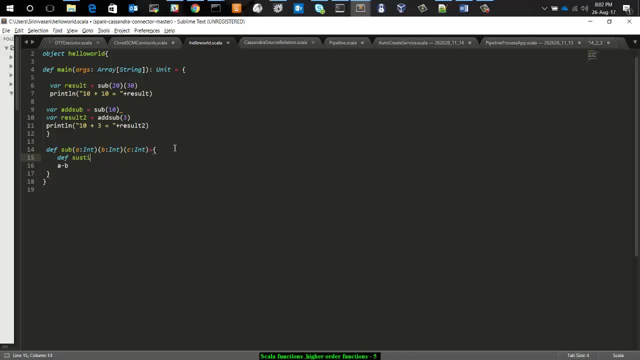 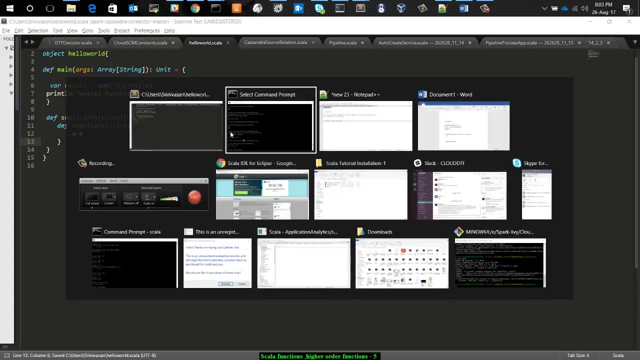 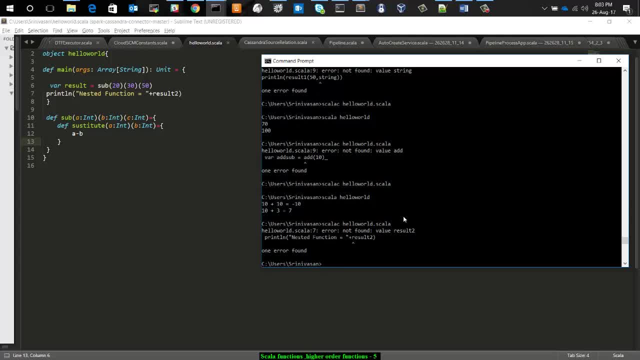 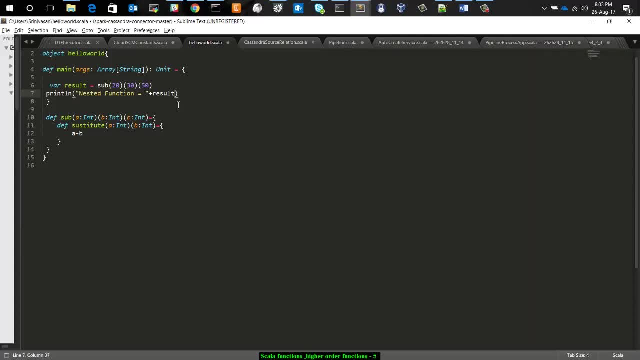 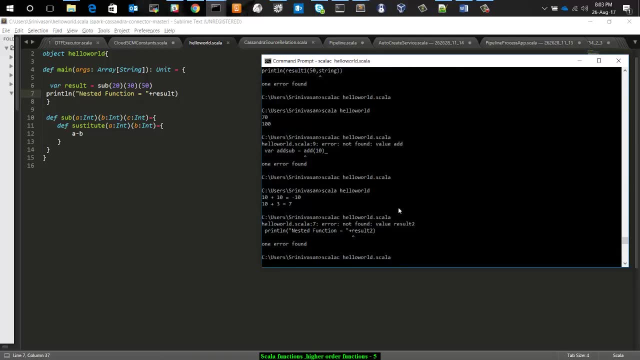 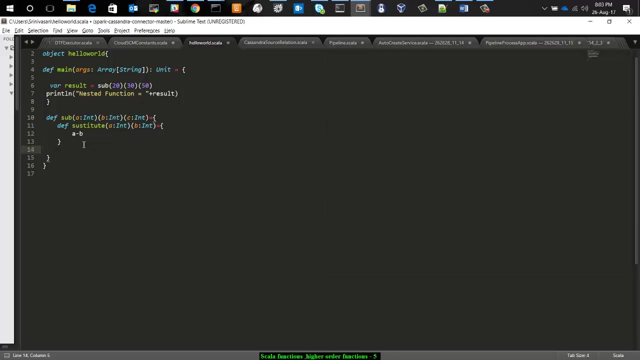 Let's see what's the output of this one shows. Okay, Let's see what it has given. It is an empty value. What's wrong with this one? We have to return the value, right? I forgot to return it here. 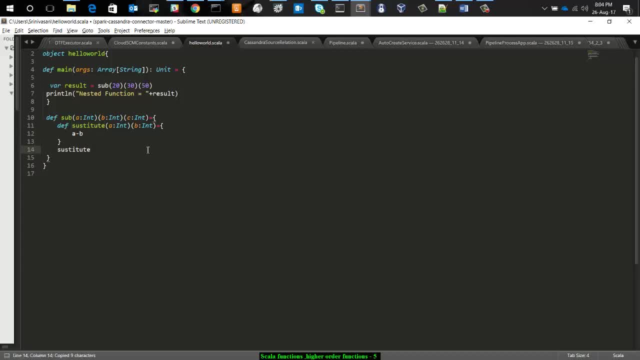 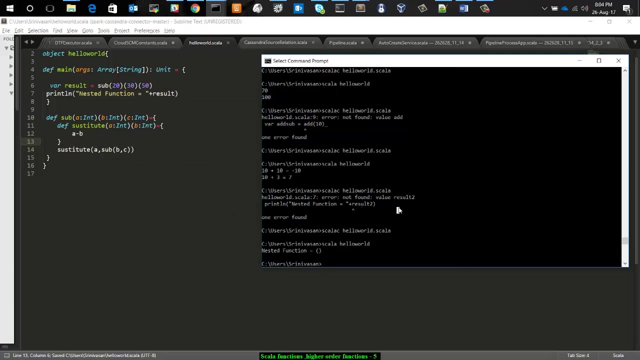 Let's see- Okay, Let's see what's the output of this one And check what it's giving. It shows that recursive method subneeds result type. Let's see what's the error in this one. It shows that recursive method subneeds result type. 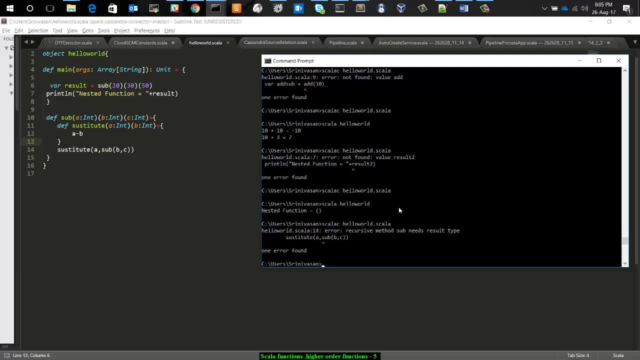 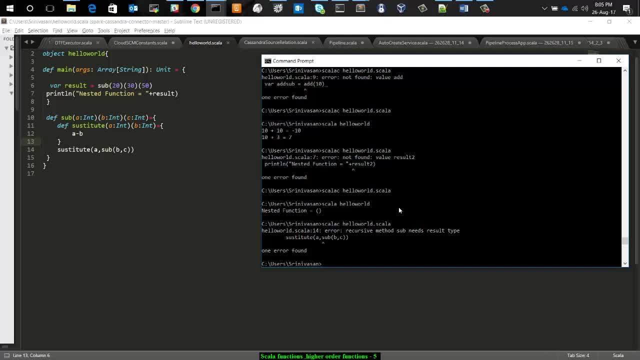 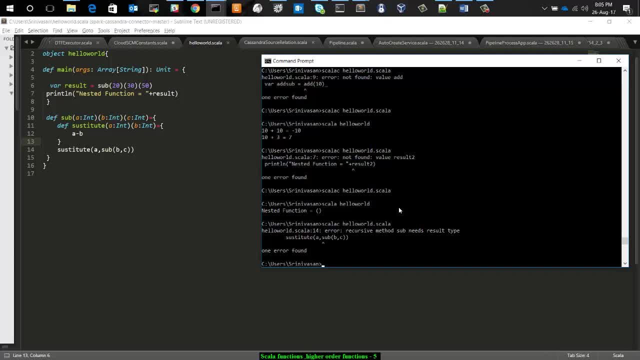 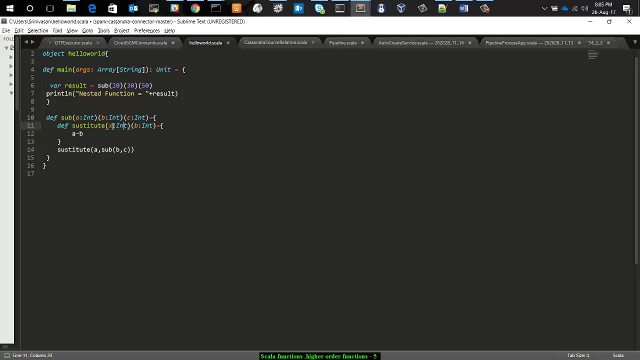 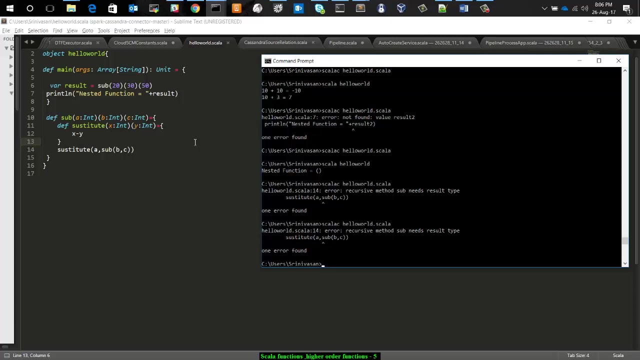 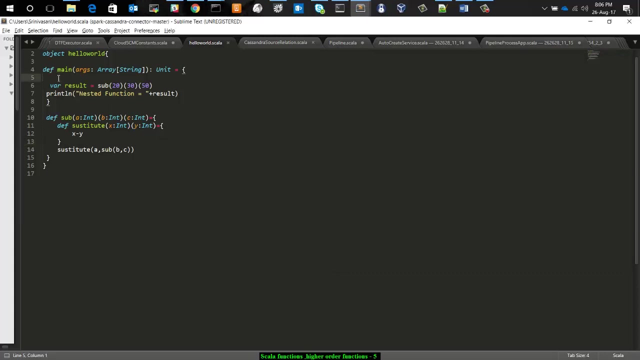 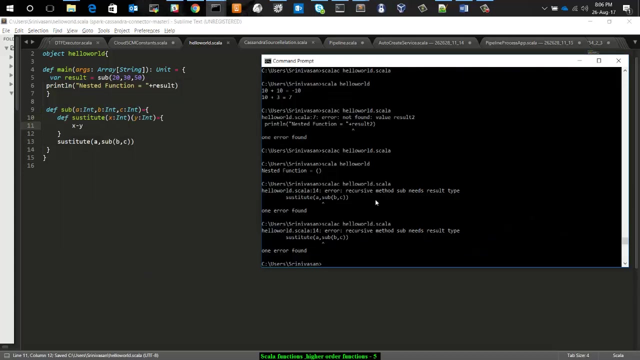 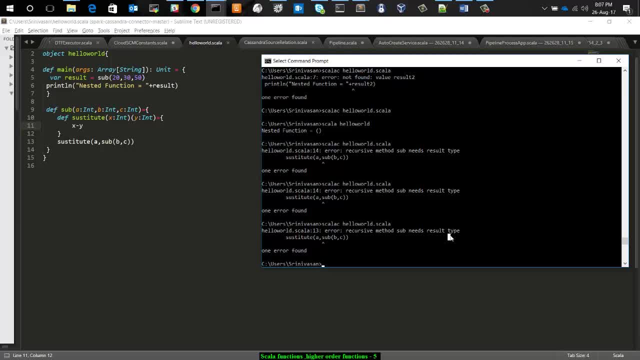 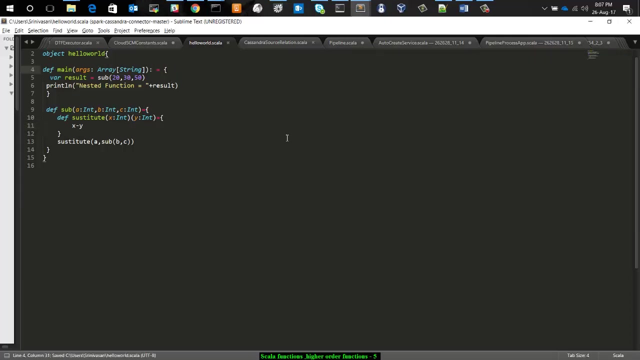 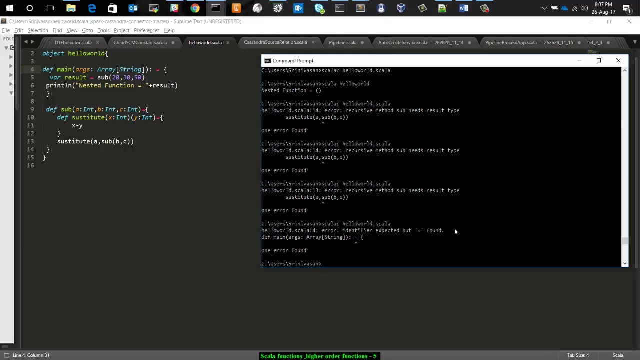 It's all the time. Let's try it again. Okay, I think this is the one that's strong. Let's try it again. Okay, I think this is the one. Come on, let's try it again. Okay, let's try it again. 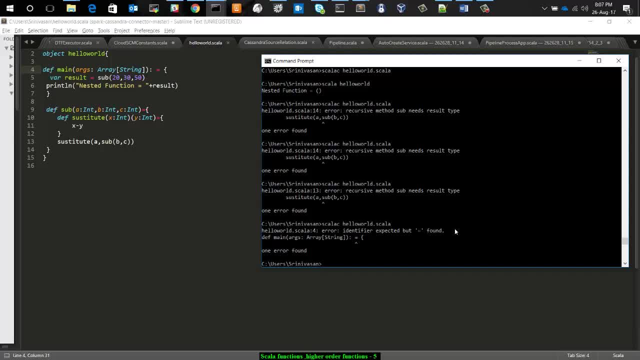 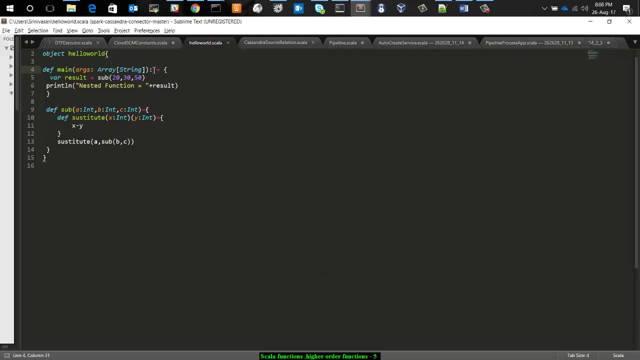 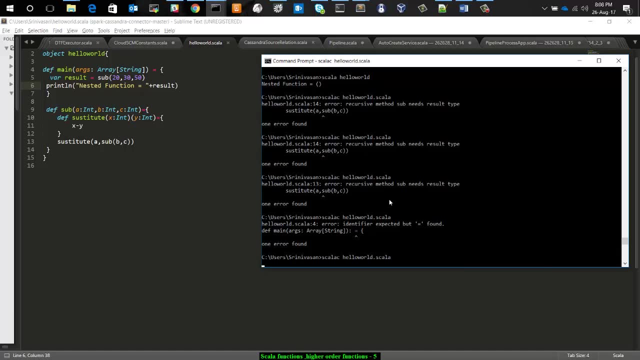 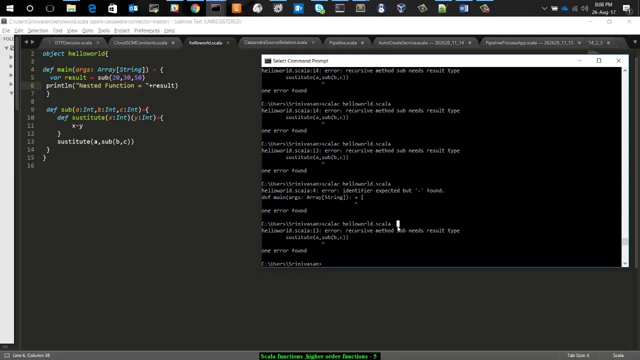 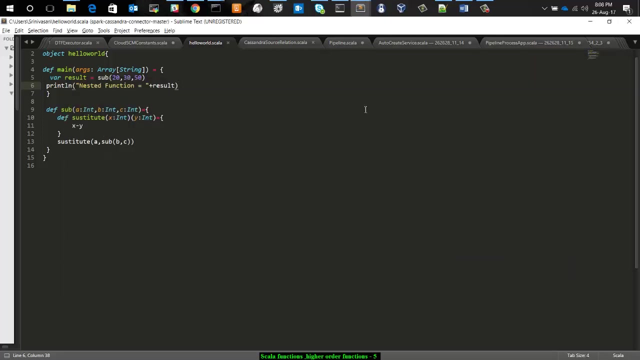 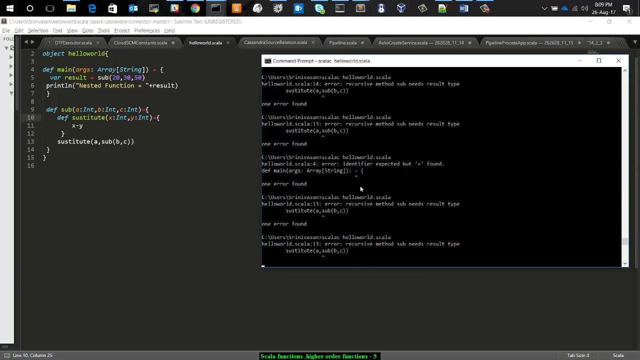 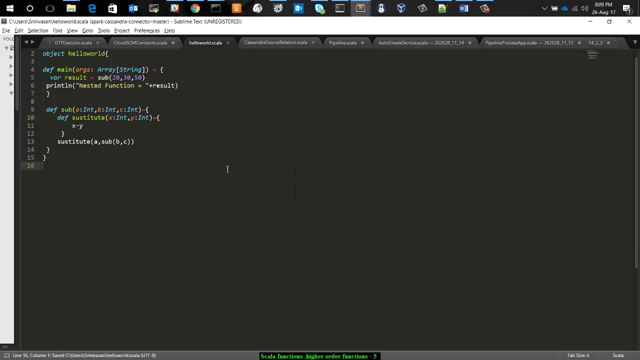 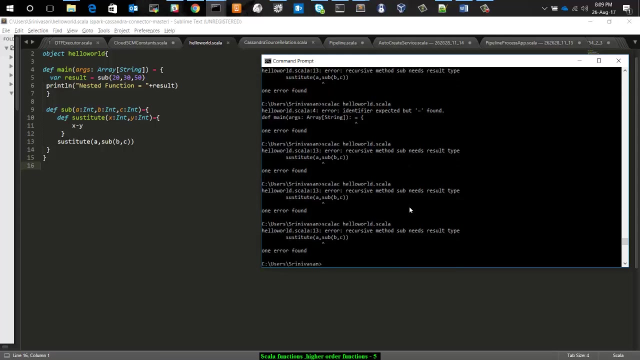 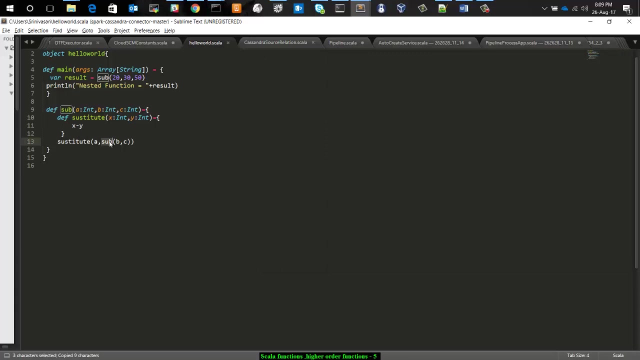 Okay, I think this is the one. Okay, I think this is the one. let's see what else we can do to take it to the right time. Okay, let's see in the mirror. Let's see in the mirror. Oh, I have called the same function over here. 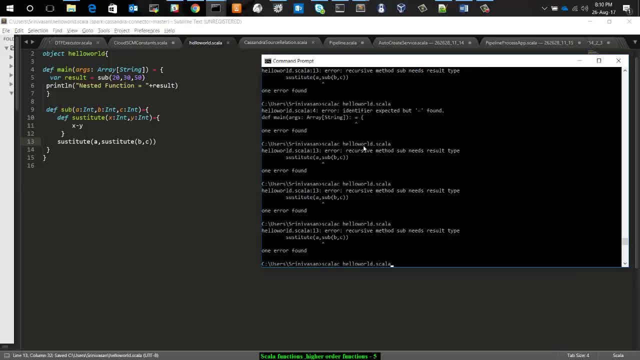 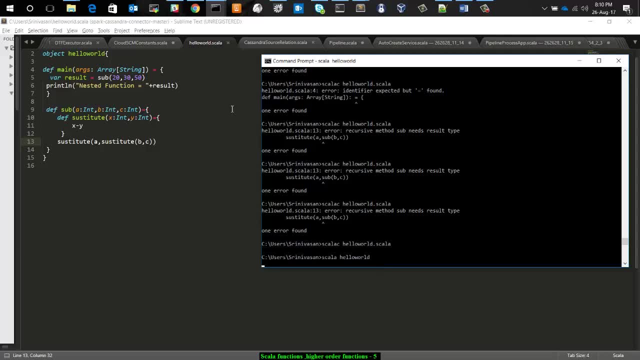 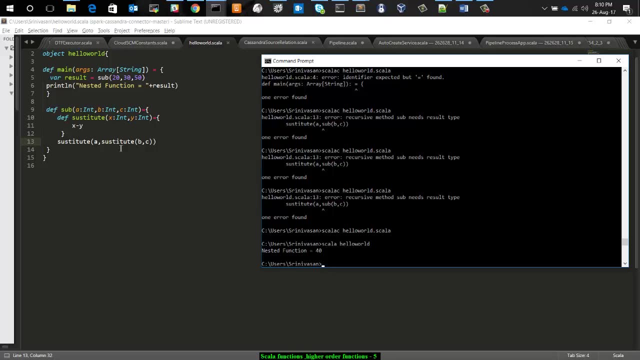 That's the thing, Let's see. I think this could work out now. Yeah, it worked. What it does is before. I am calling the same function over the recursive function, So we have to be careful while calling the nested function over here. 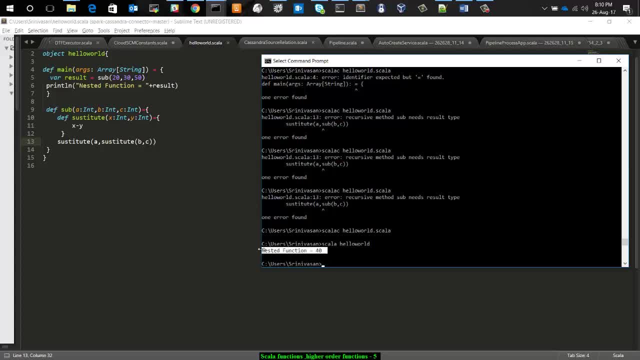 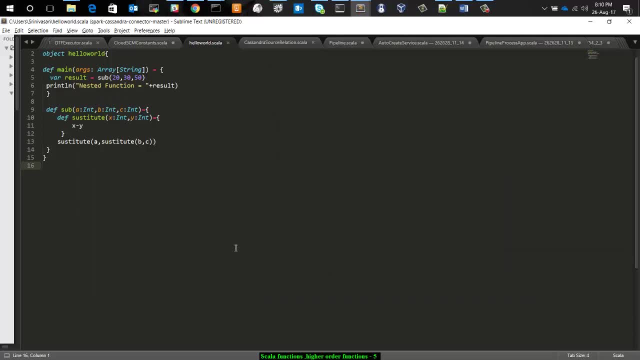 Now you can see clearly see the output which came correctly. Then in function we can see that the variable length parameters in scalar you can define function of variable length parameters. It allows you to pass any number of arguments at the time of calling. 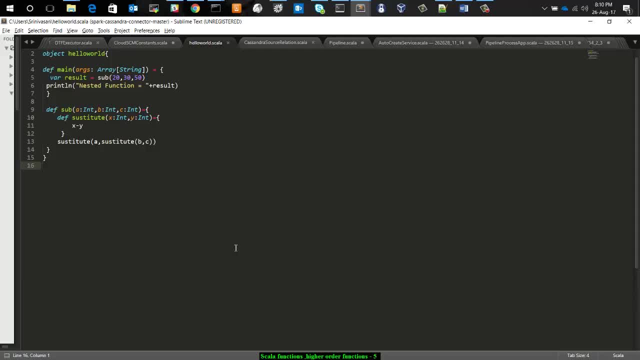 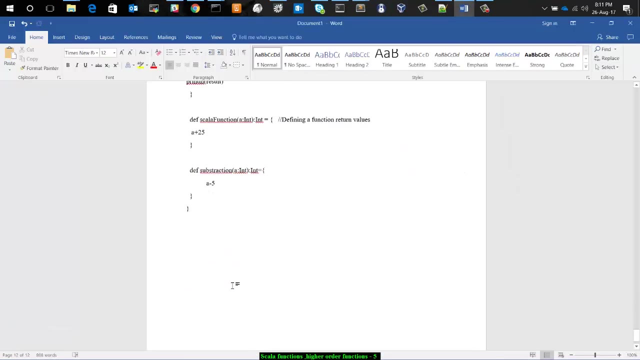 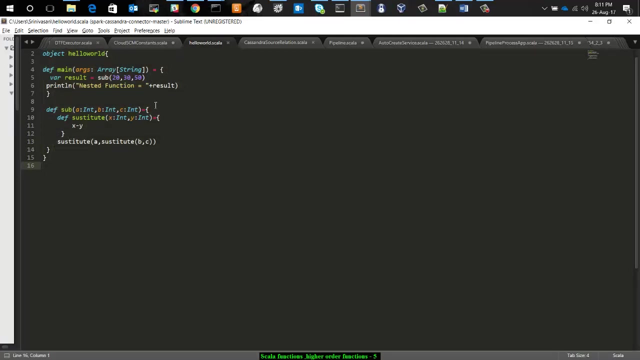 the function. Let's see one example for this function with variable length parameters. Well, it is about 1 laboratories, Let's do it. So what method does this function have to kinda calculate? It will generate the respective parameters. Then I will create terms to the function function over here in constructor. 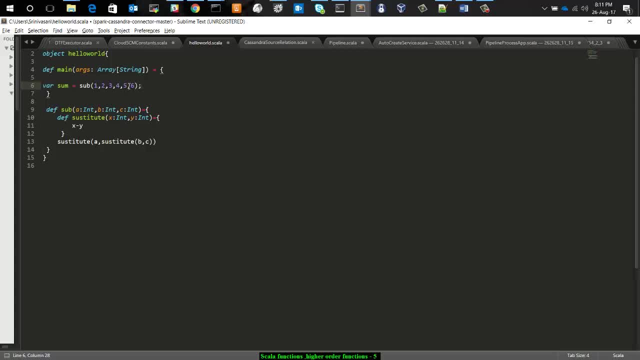 So that database under the code, So that I can somehow transform it. And that's it for this function. Thanks for watching everyone, Thank you, Thank you, Thank you. In this function what I have written is in this I am getting.